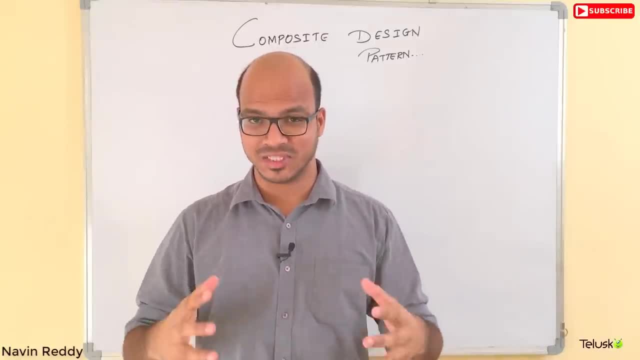 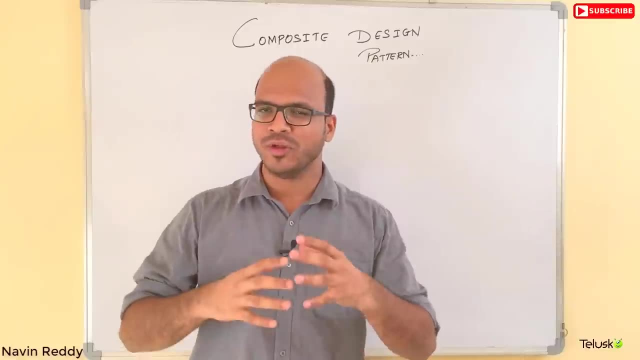 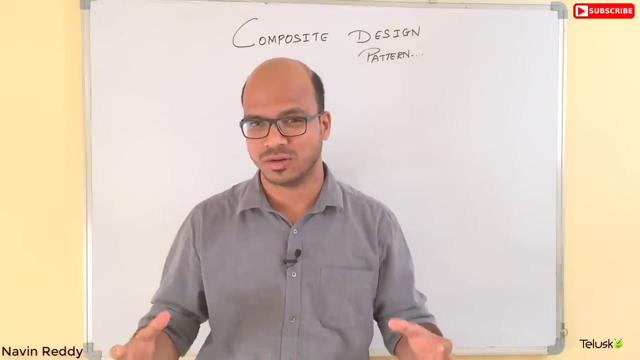 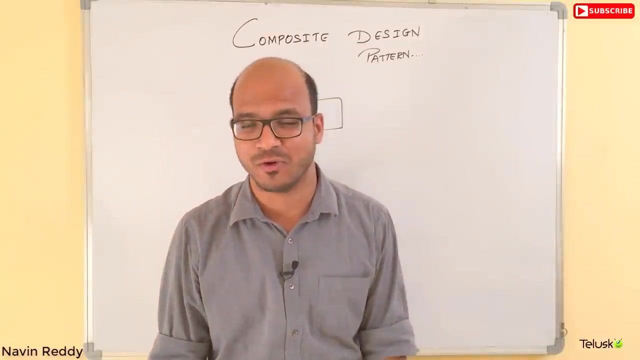 So welcome back, aliens. this is Navin Reddy from Tarisco Learnings, and in this video we'll talk about composite design pattern. Now, composite design pattern is a part of structure design pattern. So when to use this pattern? So whenever you have a scenario where you want to create object and which represent a tree structure Example, let's say when you want to assemble a computer. Now, if you remember way back, you know way back when we, when we wanted to assemble a computer, In fact, nowadays, in fact, gamers do that right, But now normal people. 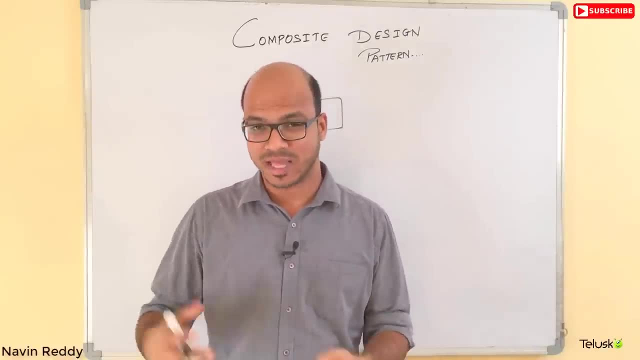 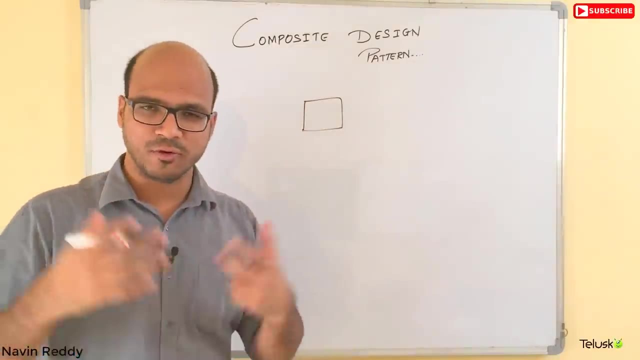 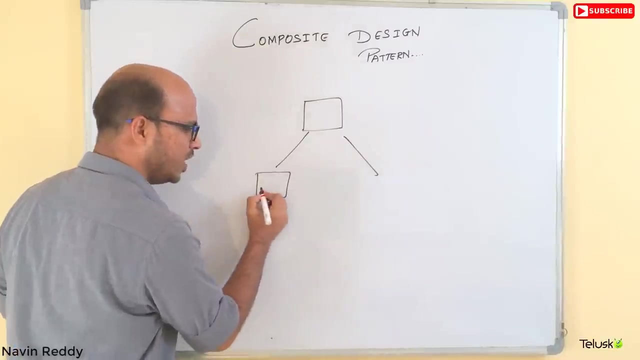 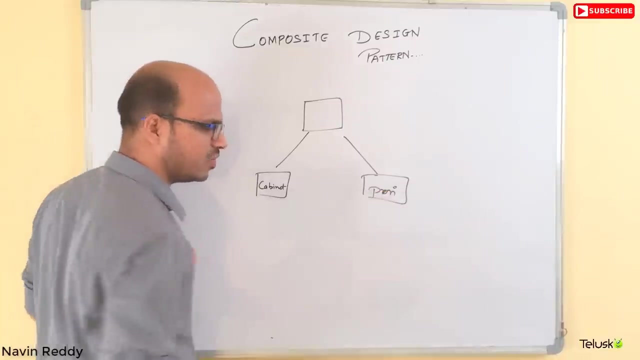 we buy laptop, we buy desktop, we don't assemble it. now, There are people who do it now also, especially gamers, people working on the server side. So let's say, if you want to, if you want to assemble a computer, what we need for a computer. So, to build a computer, we need two things: right, We need a, we need a cabinet which will have its own part, and then we need some peripheral devices. right? So we have, we need some peripheral devices. So, in a computer, in a computer, we require a cabinet and we require a peripheral device. 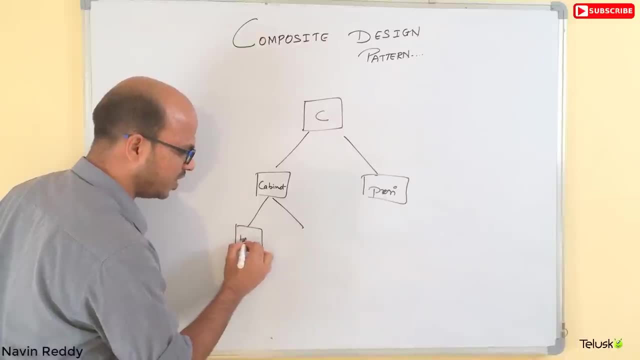 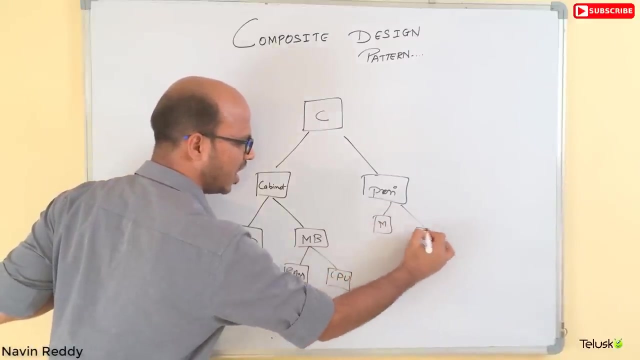 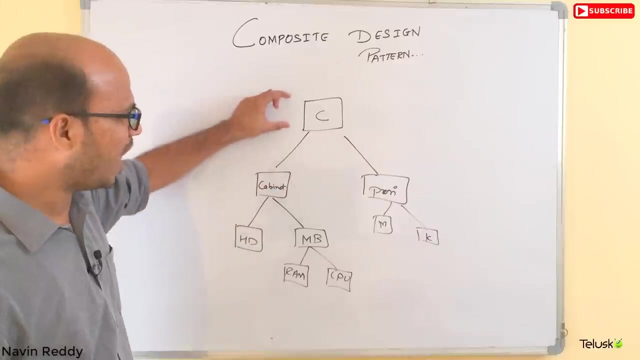 Inside a cabinet we, let's say, we need hard drive, then we need motherboard, and inside the motherboard we require- I mean, on the motherboard, you require a RAM and you need what you need- a CPU, right, And then in peripheral devices you have mouse and then you have keyboard. So when you talk about this, boxes, here, this, all are objects. right Now, whenever you have one object which has list of objects, this object will be called as a composite design pattern. 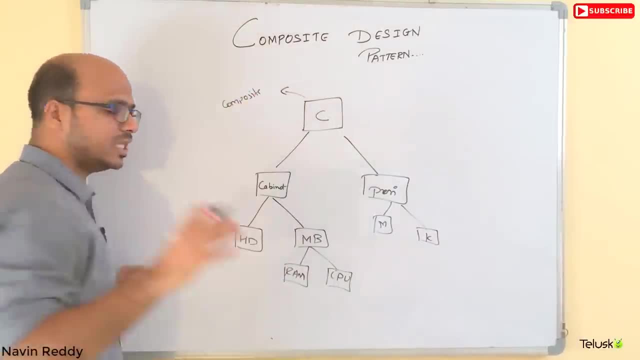 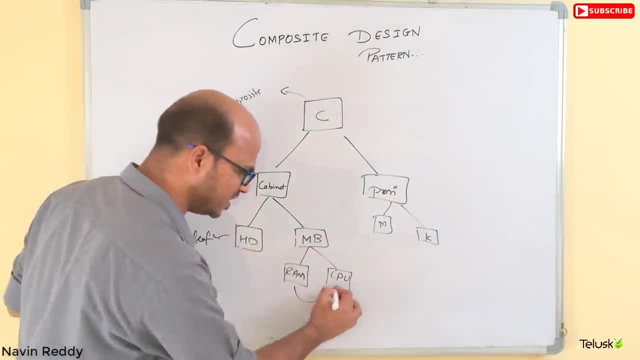 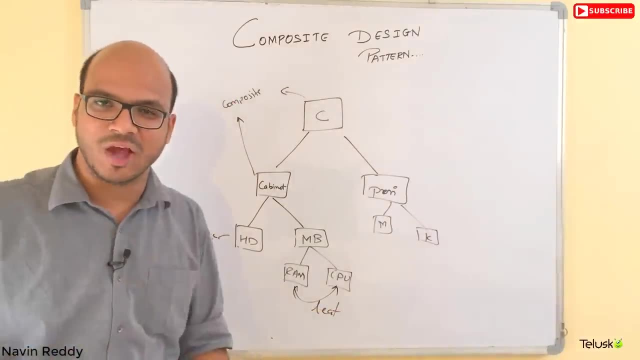 two things. here we have two more leaf objects. so this, even this, are your leaf object, right? so all this class, all these objects are of same type, right? they all are electronic device, if you want. if you talk about a computer, it's an electronic device. if you talk about a camera, it's an. 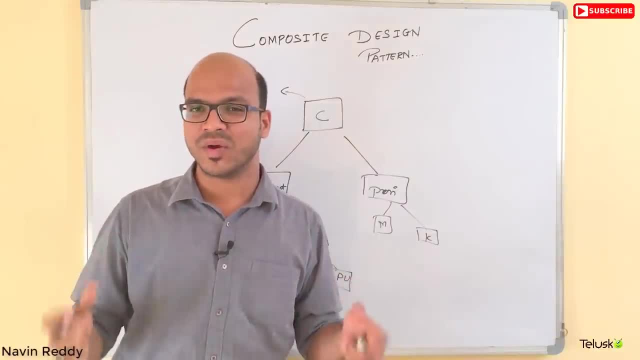 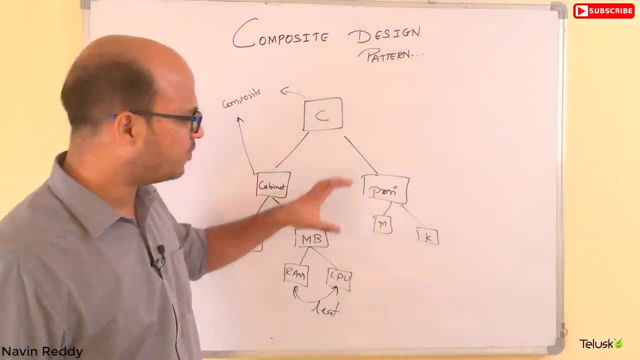 electronic device. when you talk about keyboard, it's an electronic device. that means this: they all follow same structure. they have all the same features, right, in fact we have. they are electronic device. they also have price. so if you want to buy a keyboard, you will say: what's the price of it? if 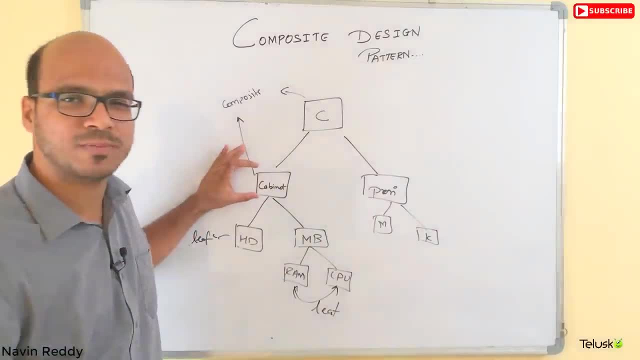 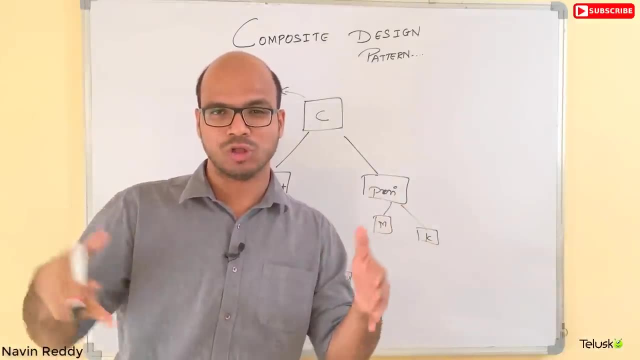 you want to buy a cabinet which has all these things, you will say: what's the price of it? i'm not talking about the, or i'm not talking about the only the cabinet structure, but the cabinet which is, which has all those objects inside that hard drive motherboard and all those things. when you 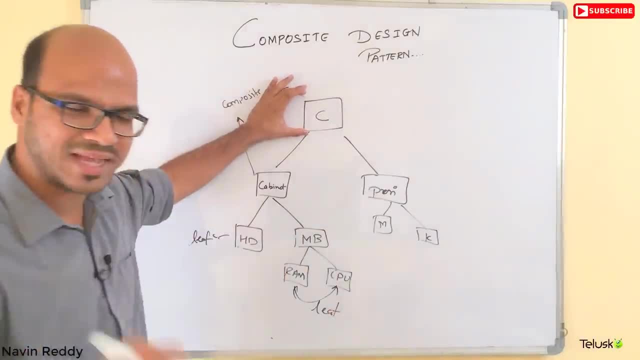 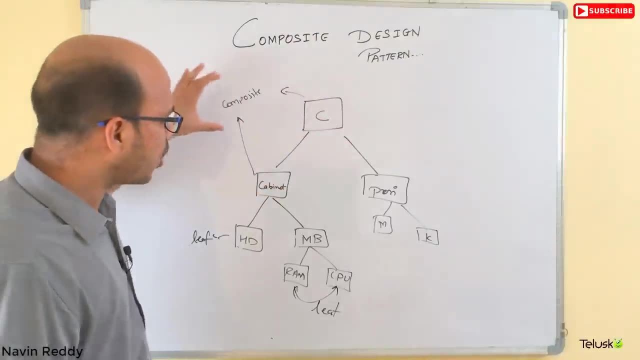 want to buy a computer, you will add all this price and you will say: that's the price of a computer, which is, let's say, any, any, any amount, right? so what is composite design pattern? is a composite design pattern will be having a tree structure where, in the tree structure, you can 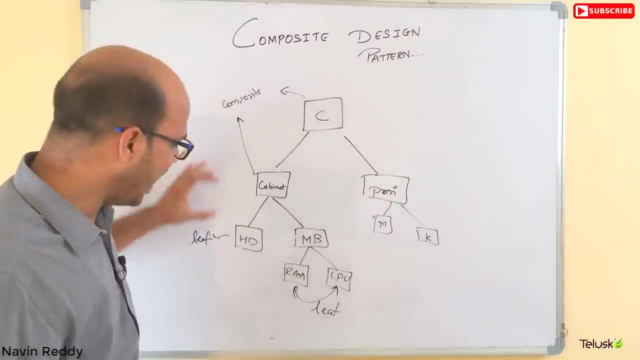 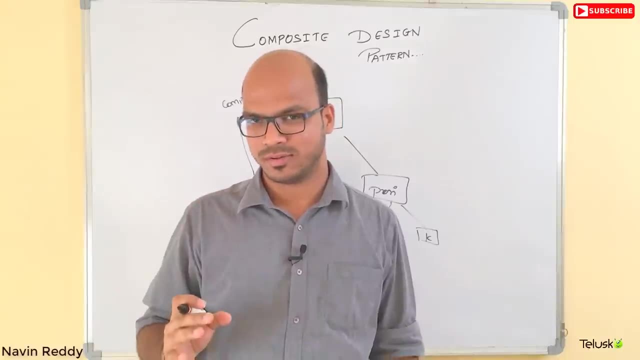 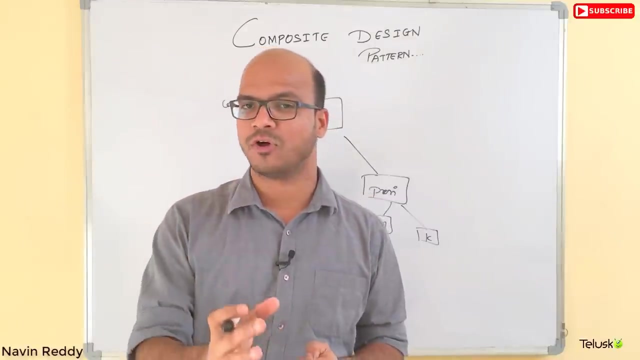 have a composite object which can have multiple objects and you can have a leaf object. now the funda here is if you can perform certain operations on leaf node. let me repeat: if you can perform some operation of lee on leaf node, the same operation need to be performed. 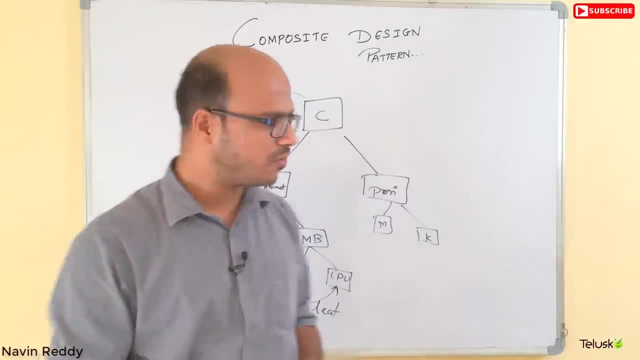 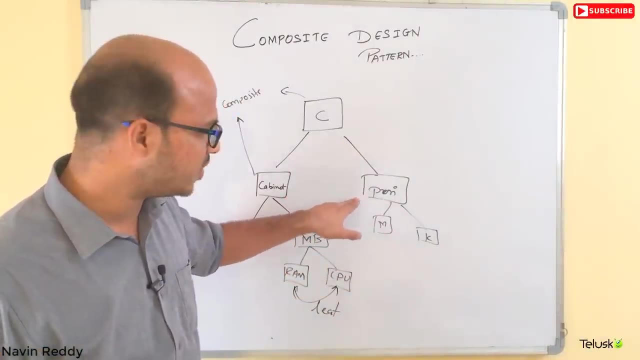 on the composite object or composite node. example, if i want to get the price of a keyboard, i should also be getting able to get the price of a peripheral device. if I want to get the price of a peripheral device, I should also be able to get the price of the 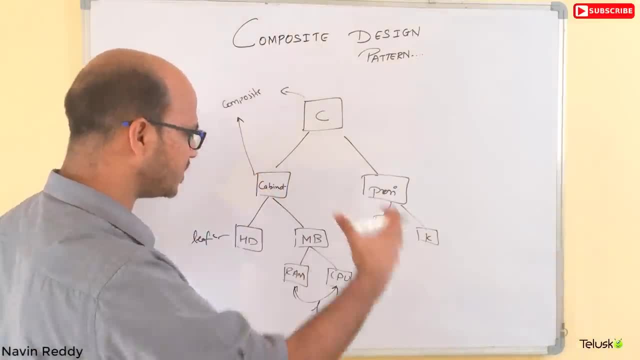 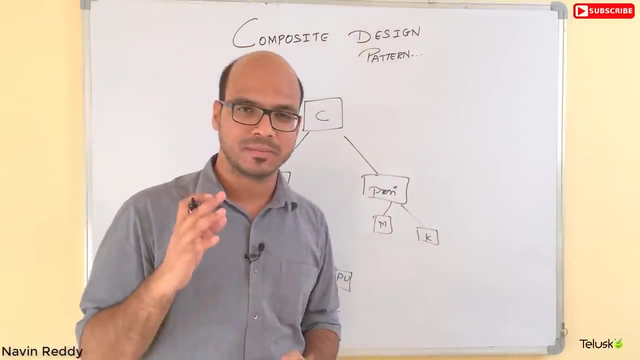 computer right. so if you want to, if you want to create something like this, that's that's where you use composite design pattern. again, how to implement this, that we'll see in the practical video. but remember this thing: composite design pattern is used where you create a object, structure or a tree, or you. 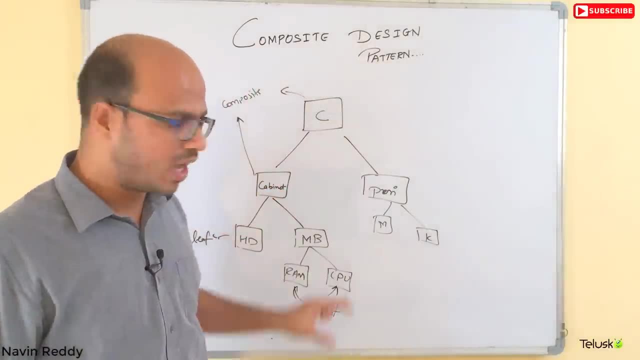 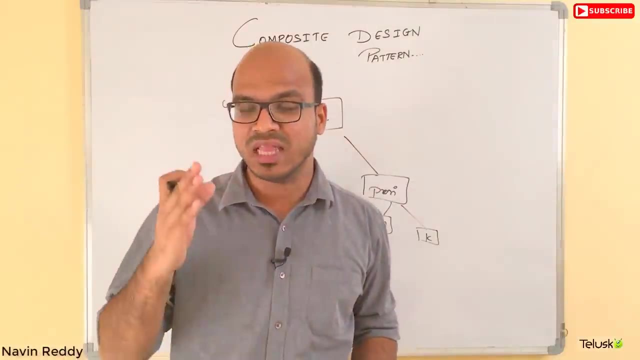 create a software in a tree structure where one object can have multiple objects and that object can have multiple objects, right, and whatever operation you can perform on the leaf node, the same operation should be performed on the composite object as well. okay, so that's it on this video. we